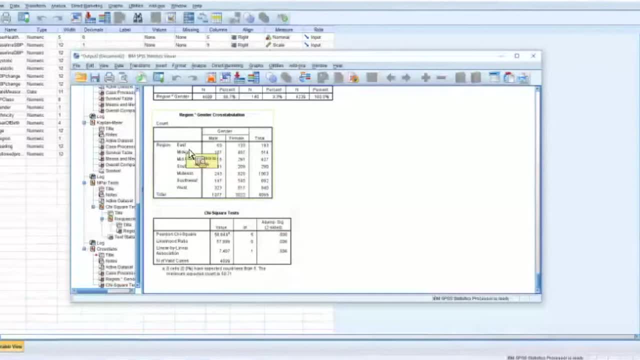 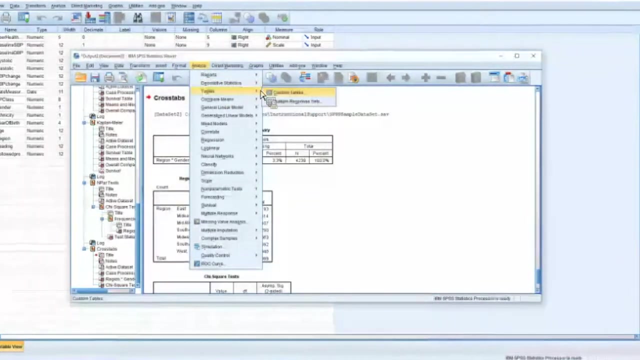 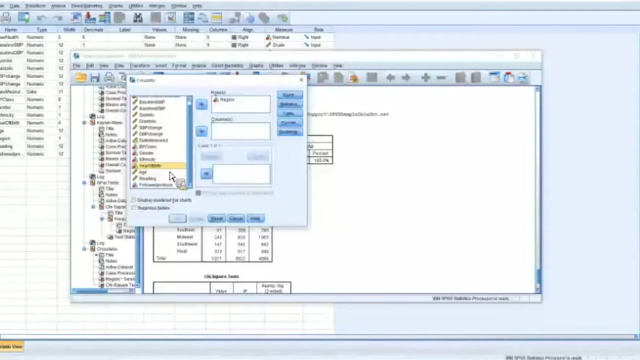 And it's looking at again. these are looking at the frequencies, So it's not looking at the mean blood pressure. It's looking at the number of people in each of these regions by their gender. The cool thing with the cross tabs is you can do it, doesn't just have to be two groups So we could have region by their blood pressure. Oh, let's do it by ethnicity. It's going to have a much bigger 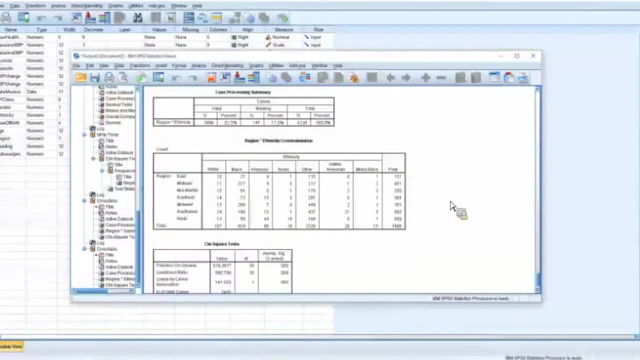 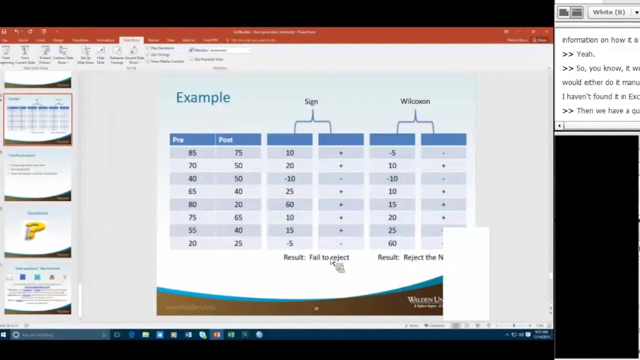 That would be interesting. So now you've got the different regions by the different ethnic groups represented in this data set. Then we have a question They're asking: can I use non-parametric methods for data collected using a Likert scale? What there's a typo here, data I guess they're using, or what type of data for a true-false answer? Well, that's categorical. So I would assume yes. 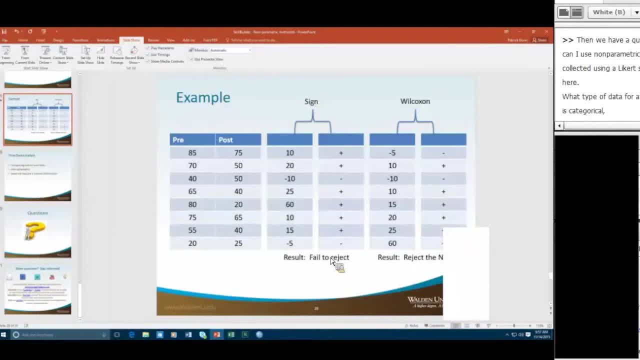 Yeah, Yeah, If you're using a Likert scale, if you're using true-false, that's exactly when you would use a non-parametric method, Right. 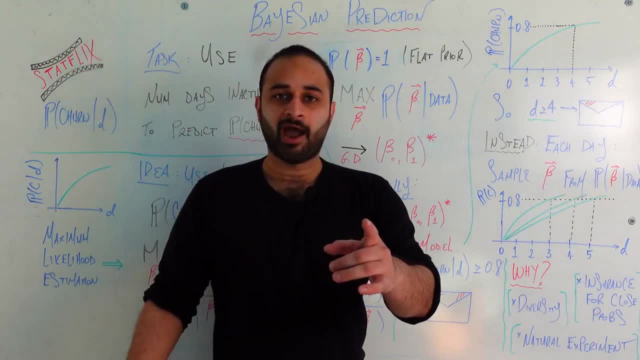 Hey, everybody, welcome back. So most of the videos on this channel we're talking about some kind of specific data science or machine learning concept and doing a deep dive into that concept In this video. instead, I want to take a step back and look at the whole. 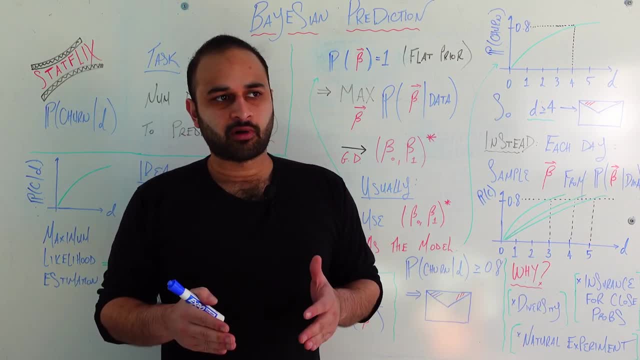 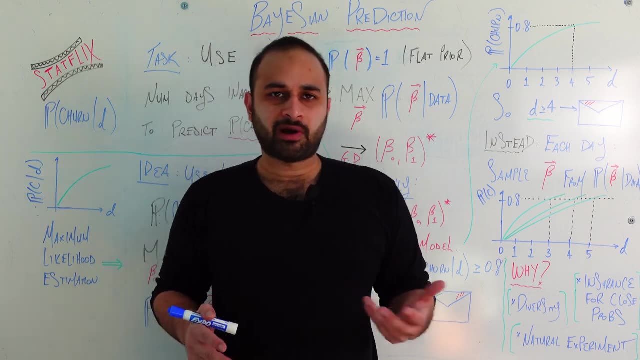 pipeline of machine learning and specifically focus on the part near the end of the pipeline where we're making predictions using some model that we've trained. Now, the typical way we think about the pipeline is: I have some training data, I use it to train some. 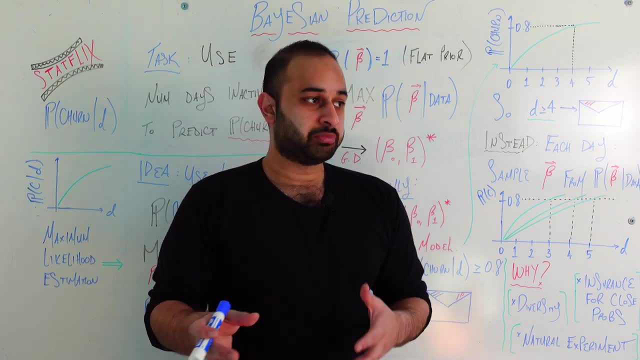 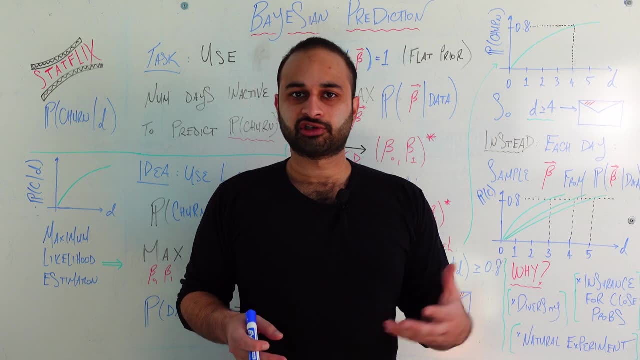 kind of smart model. and then I use this smart model to make predictions about my problem, whether it's a classification or regression or whatever kind of problem it is, and I just keep this model around until it's not doing a good job anymore. I want to kind of fight. 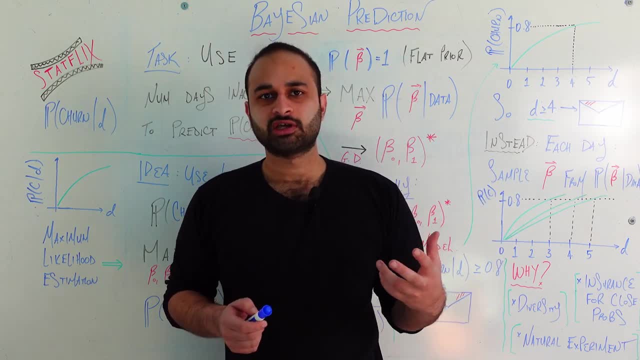 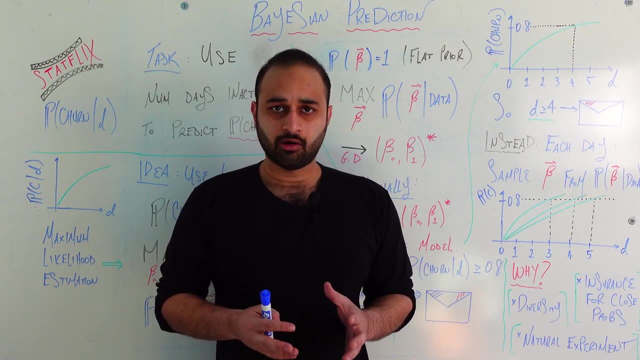 that notion kind of think about a different way of doing predictions that's more in line with Bayesian stats or Bayesian reasoning, And so that all sounds a little bit abstract right now. so let's dive into a real world example to explain this point. So we've used